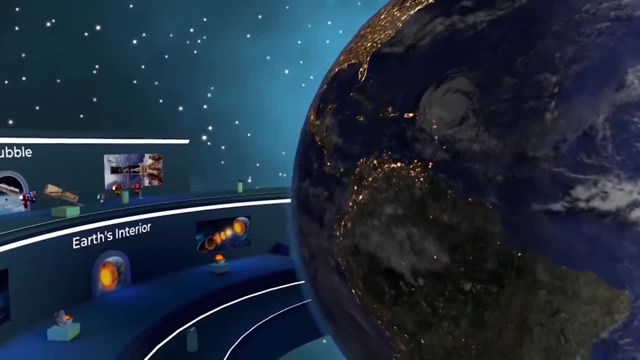 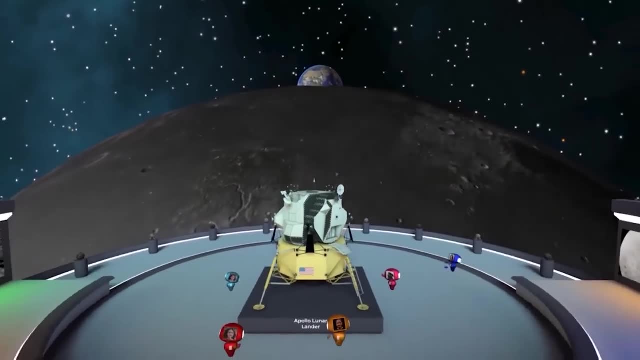 no other. Learn about astronomy while navigating through awe-inspiring environments that showcase the solar system, its planets, their moons and other solar bodies. Enter the planetarium to discover mind-blowing images, videos and models, all rendered in stunning detail with audio. 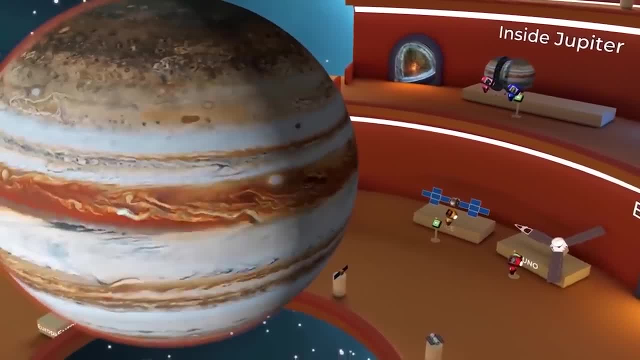 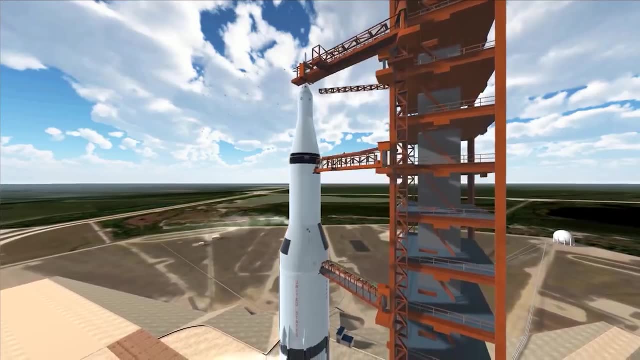 descriptions, toys and more. If you're interested in learning more about the planetarium, please visit the link in the description. I've never personally used this one before, but I have heard good things about it and since it's free, you can always give it a shot. Number four: Apollo 11.. These last two space experiences are 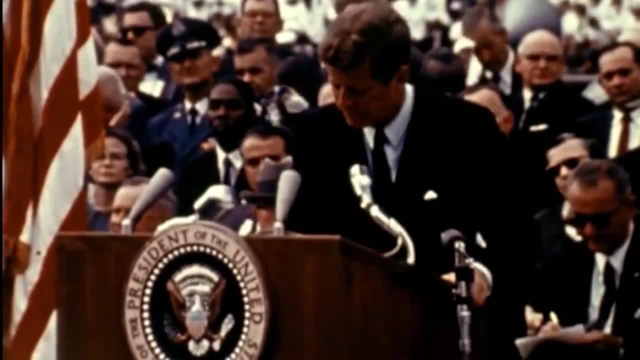 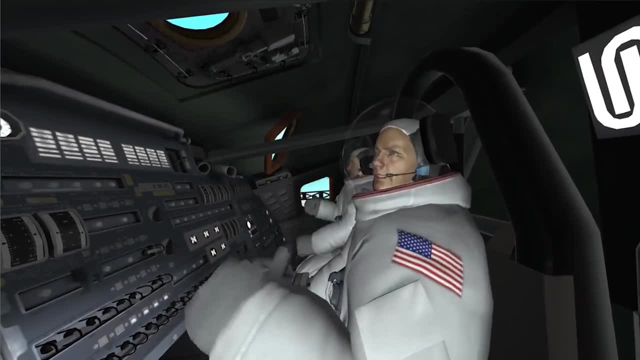 very different from the others. You'll get the chance to experience the historic events of Apollo 11 from the perspective of those involved with the mission. It's a pretty surreal experience that really allows you to see the events from a new perspective and it works great to teach about. 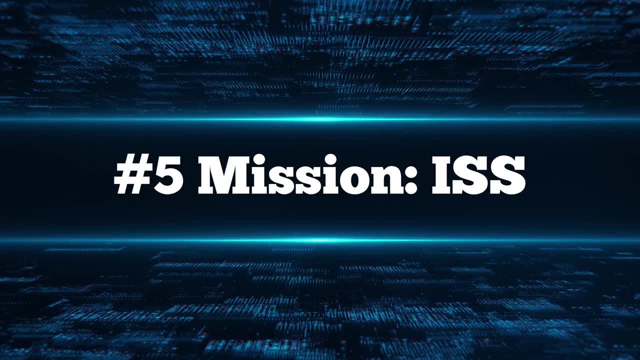 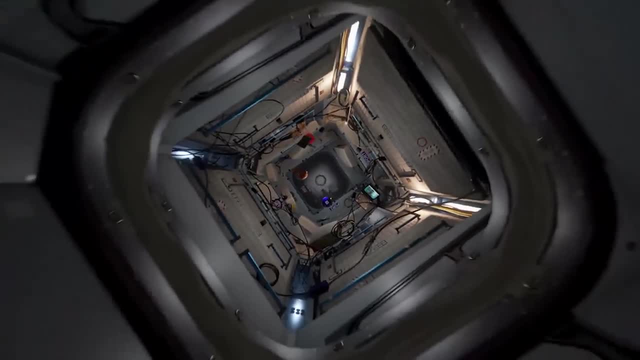 history and space travel. Apollo 11 is $9.99.. Number five: Mission ISS. The next experience is one of the most amazing free experiences on the quest, and that is Mission ISS. In Mission ISS, you get to visit the International Space Station, float around in zero gravity, go out into space. 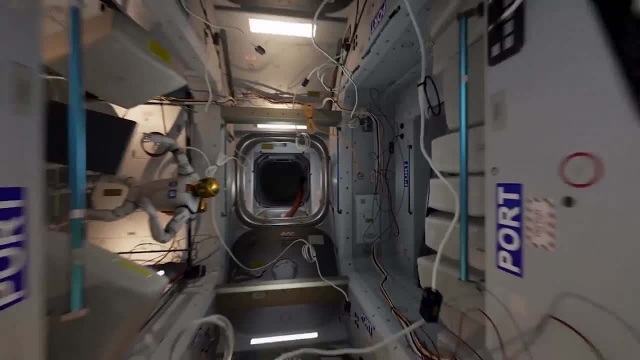 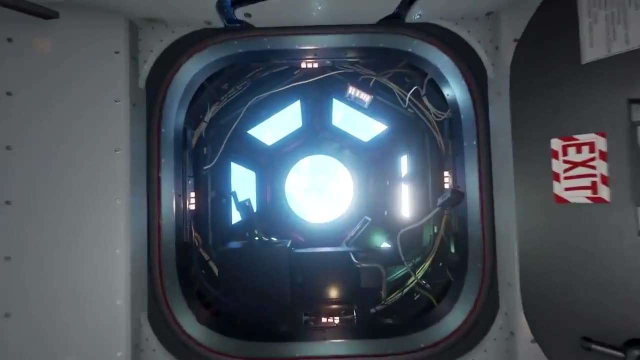 on a spacewalk and even help perform certain tasks on the ISS. This experience is as close to being up in space as you can get in VR, and it's a great educational tool to show how those on the ISS live and go about their daily lives. The only thing to keep in mind with this experience is that 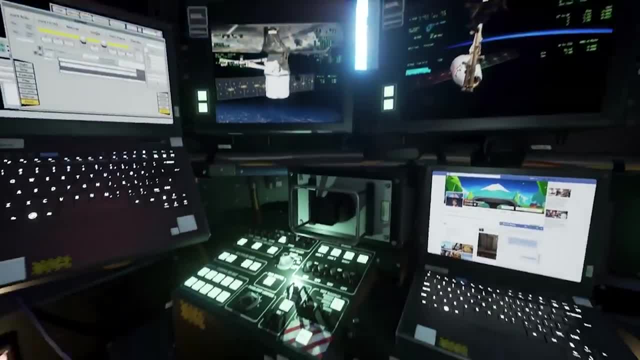 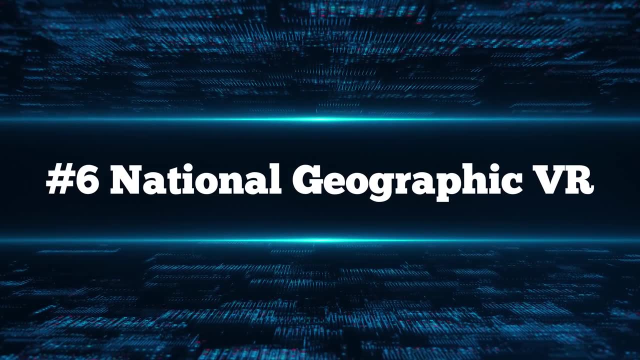 due to the zero gravity nature of the game, it can cause some motion sickness in some people, so just keep that in mind. But for free, Mission ISS is just stellar Number six. National Geographic Explore VR- Well, we've talked about space. 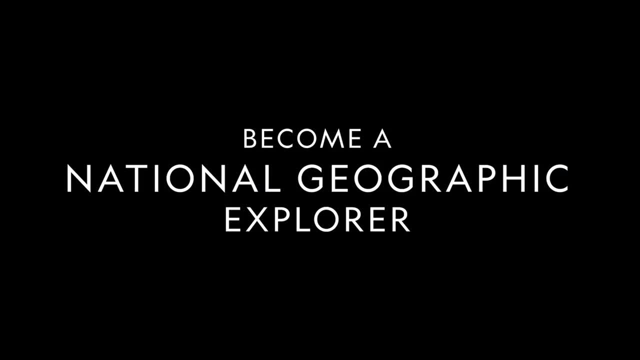 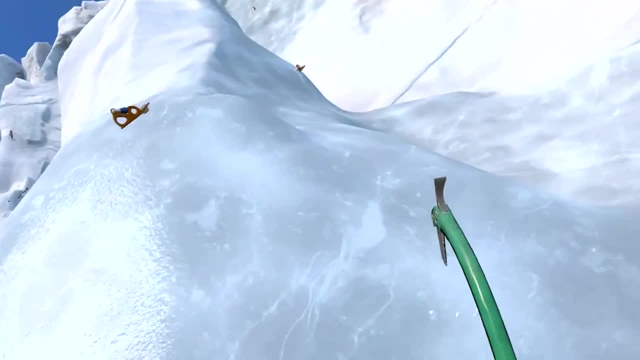 now let's talk about our planet with some history and geography experiences. National Geographic Explore VR is still one of my favorite experiences on the quest to show people the power of travel and learning. Right now, there are two places you can go In Antarctica. you will kayak. 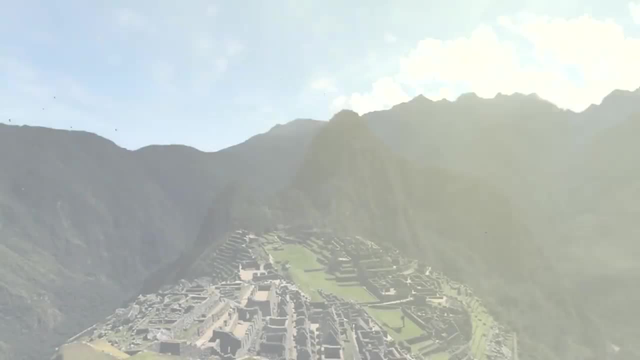 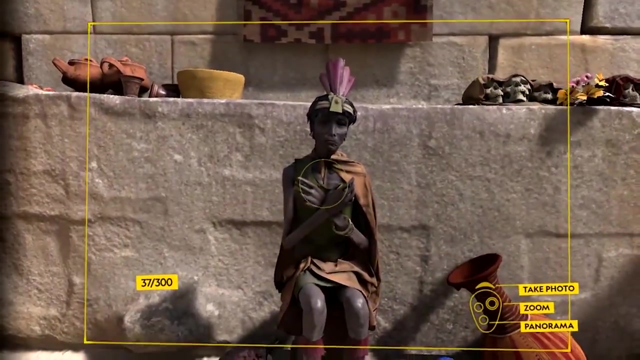 through the icy waters as whales swim underneath on the search for penguins, Take pictures and climb an ice wall in the stunning experience. Then, when you're done, Machu Picchu to explore the ancient ruins as you take photos and step back in time to see what it 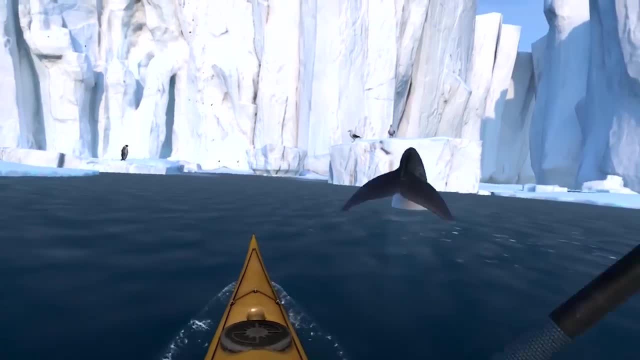 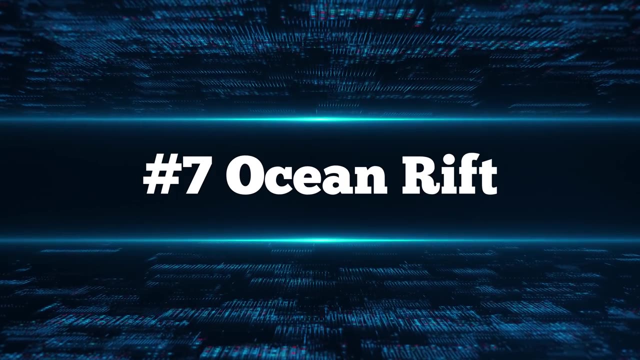 was like to live many years ago. My 10-year-old son loves this game and I can feel good knowing that he can learn while also enjoying seeing the world. National Geographic Explore VR is $9.99.. Number seven: Ocean Rift. Now it's time to head under the ocean and explore In Ocean Rift. 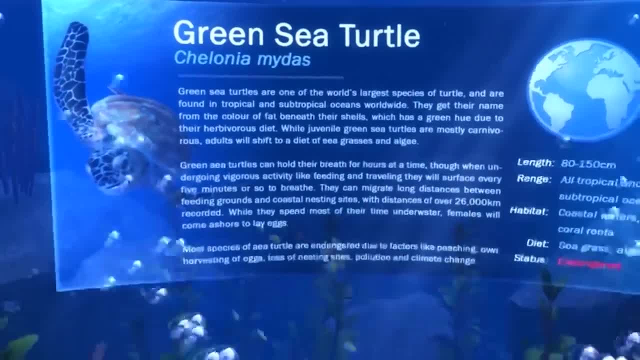 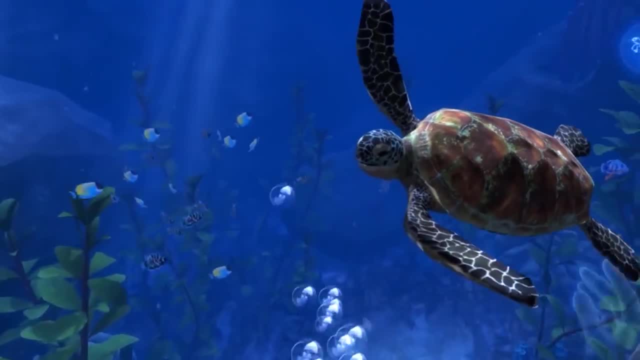 you can freely swim around 14 different habitats full of living creatures. You can see dolphins, sharks, whales and so much more. For those who love animals or learning about them, this is an amazing opportunity to swim with creatures you would otherwise never see or want to see in person. Plus, if you activate education mode, 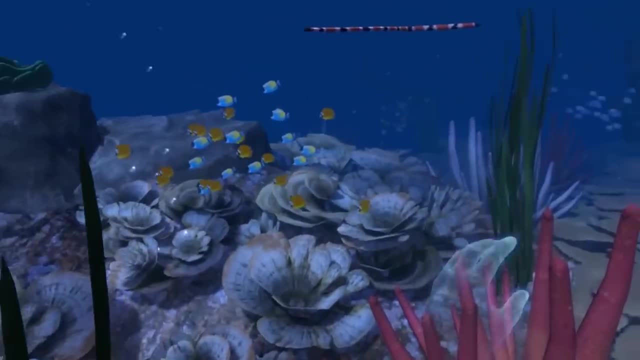 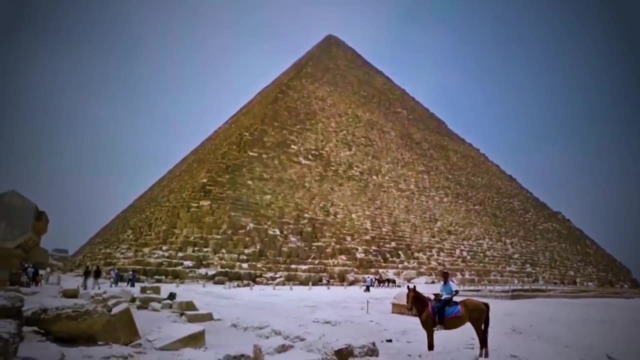 there are over 40 narrated education points. you can find teaching about the creatures and their habitats. Ocean Rift is $9.99.. Number eight: Wander. Now that you've explored some 3D renders of the world, let's explore the real world. In Wander, you can travel all over the world and 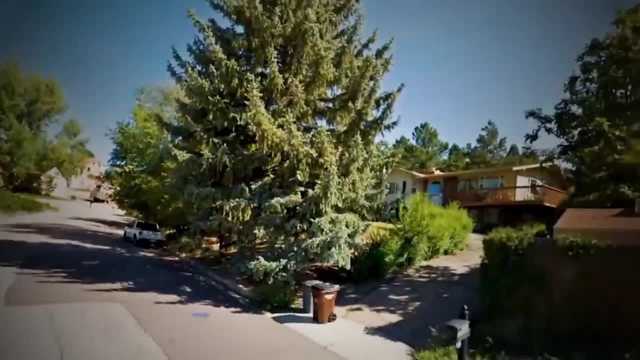 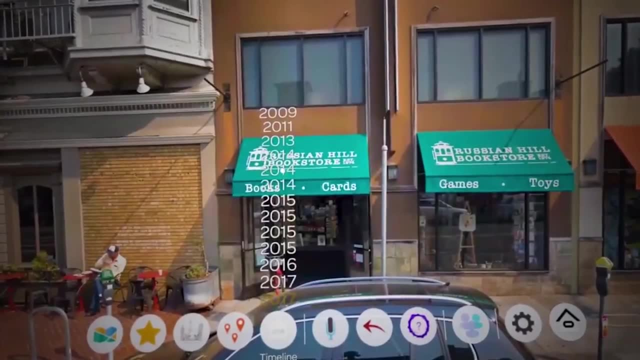 see the sights, visit locations you've only ever dreamed of, or step back in time and check out some locations from your past. This application uses Google Street View and photos to create an experience that allows you to jump from locations you've never dreamed of. You can also explore the 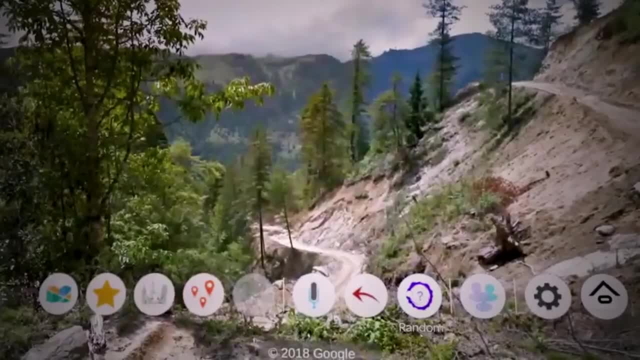 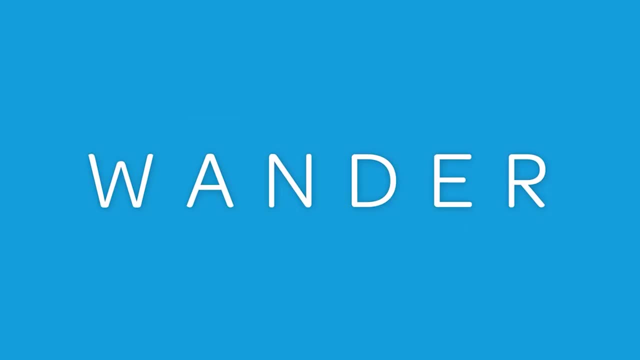 world from location to location and see them in full 360 degrees. It works great as a travel experience to see the world or if you're learning about a specific place, you can jump there so you can better visualize what it looks like. There is even Wikipedia integration for additional learning. 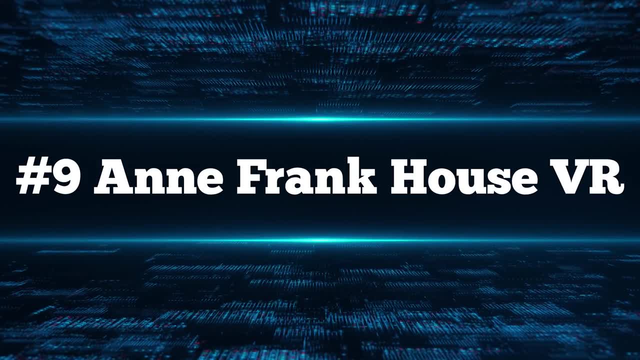 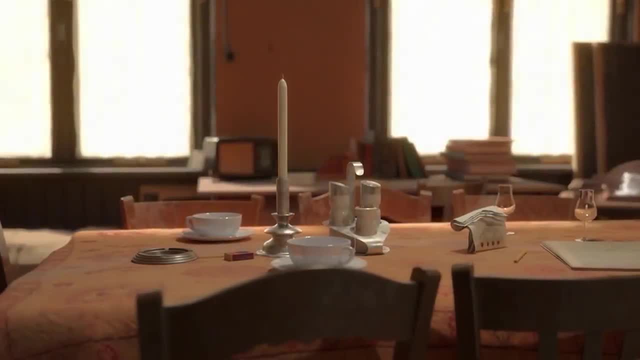 Wander is $9.99.. Number nine: Anne Frank House VR. History has always been one of my personal favorite things to learn about, and this next game shows the beauty of VR and learning about history. In Anne Frank House VR, you get to explore the childhood home of Anne Frank during the World. 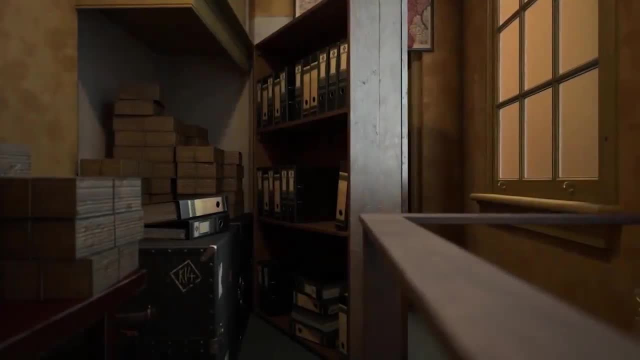 War II era. You can explore the world of Anne Frank. and you can explore the world of Anne Frank during the World War II period. Enter the secret annex and see where Anne and her family hid to escape from the Nazis. This experience is amazing, with a narrated tour of the house as well as the 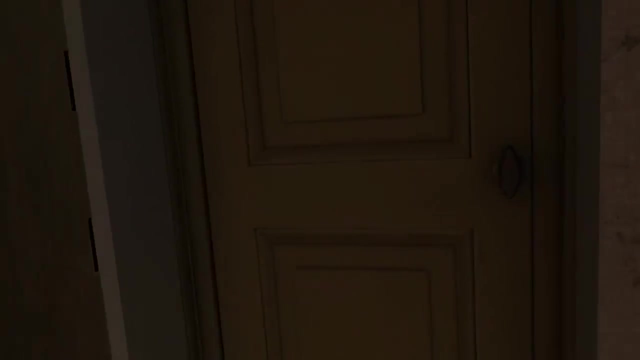 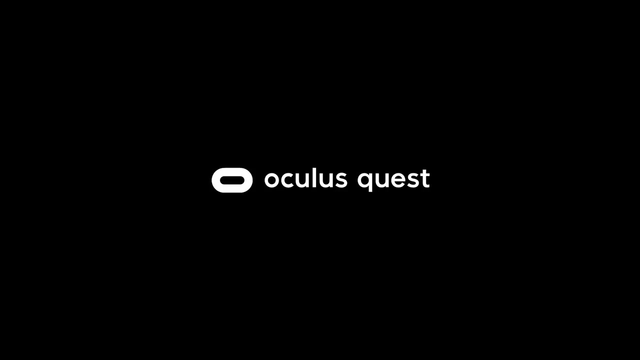 ability to just explore and look around. It helps to really bring history to life in a totally new way. Anne Frank House is free. Number 10, Beat Saber. Why is Beat Saber on this list? you ask? One thing all people, including kids, need is physical activity and being stuck inside. can. 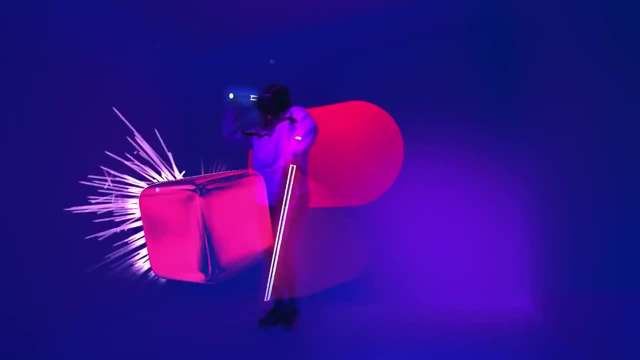 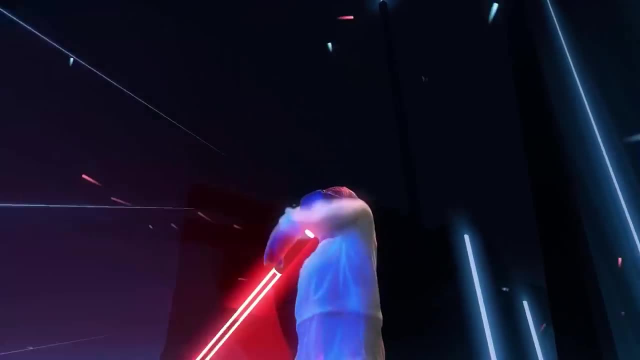 put a damper on that. One way to fix that is to use some of the awesome experiences on the quest to encourage getting up and moving. The first of those games is Beat Saber. Slash the cubes to the beat as you swing and dance to the musical tracks while also feeling like a Jedi. Beat Saber is. 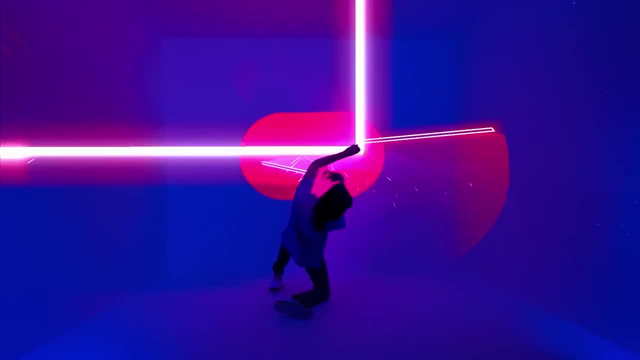 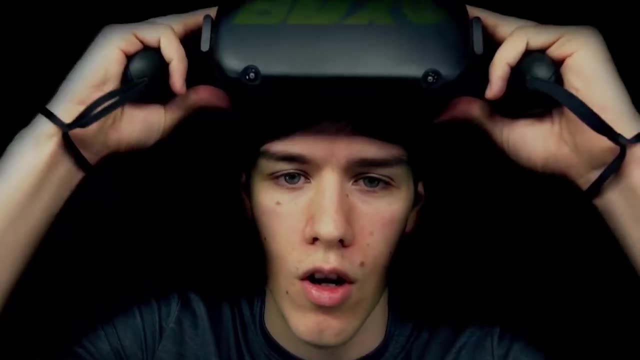 probably the most well-known music rhythm game in the world at this point, and if you're looking for physical activity, you can't go wrong with it. Beat Saber is $29.99.. Number 11,: Box VR. If you're looking for a more structured exercise, then Box VR is for you. Box VR is designed from. 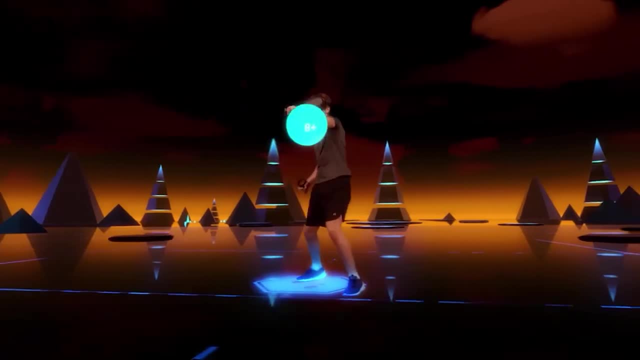 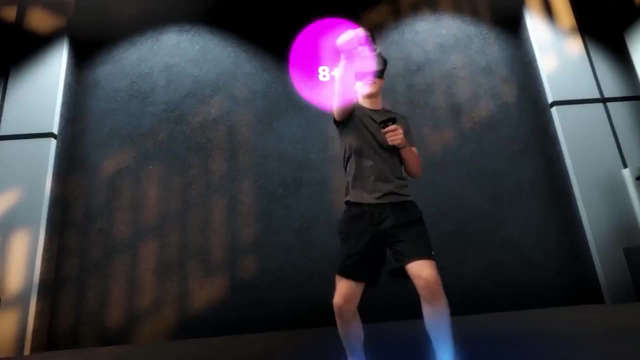 the ground up to be a cardio and exercise experience where you can pick from a list of workouts at different lengths. This game is great for getting your heart rate up and encouraging movement and exercise. Box VR is $29.99.. Number 12, Synth Riders, Last on our list of games to get you up. 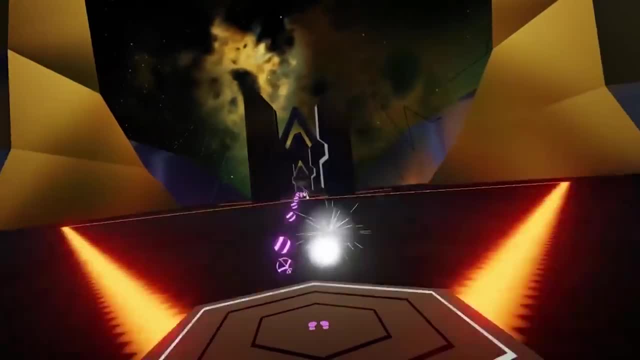 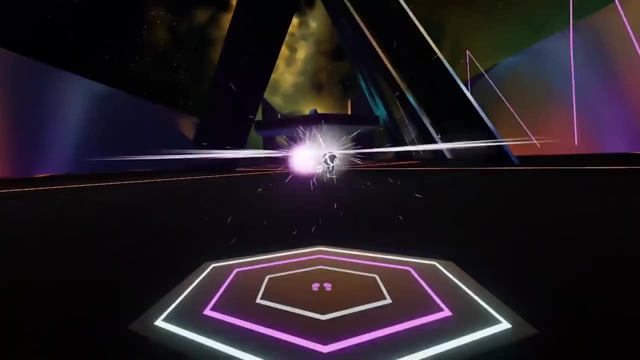 and moving is Synth Riders. This game is a little more calm than the other two, but don't let it fool you, It's still an incredible workout. Dance to the music as you move your hands to hit the proper targets. This game is a lot of fun and will get you up and moving around while having a grand. 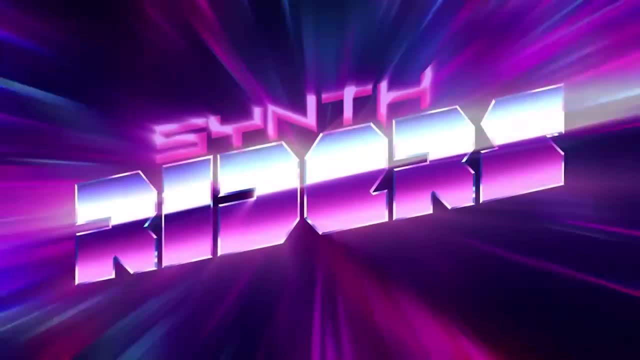 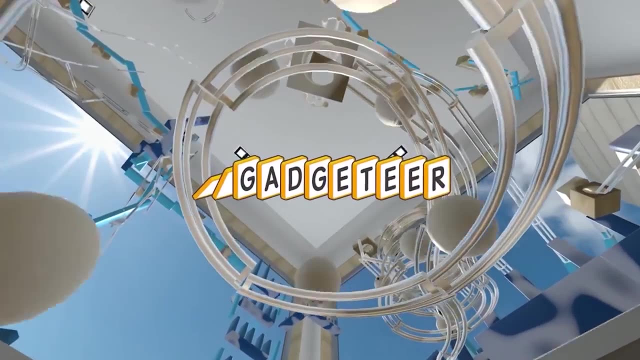 time listening to great music. Synth Riders is $19.99.. Number 13,: Gadgeteer. Now that we've worked out our bodies, let's work out our minds. Gadgeteer is an amazing game that gets your mind working hard to solve puzzles using physics. This game encourages not just learning. 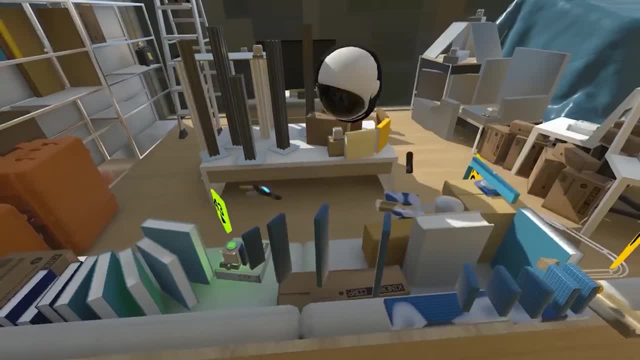 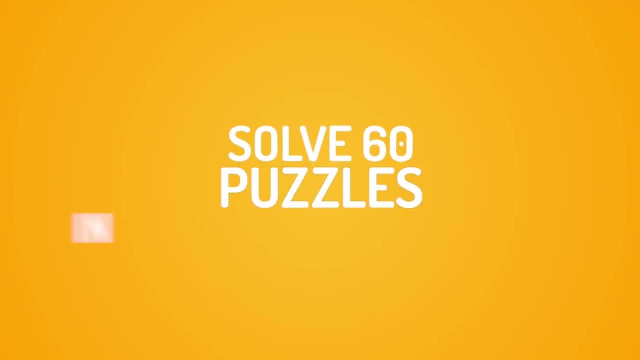 about how physics work, but also problem solving, and it's just a great way to flex your brain muscles. Then, if you really want to get your mind working, start creating your own puzzles. That'll really get you thinking about physics and mechanics. Gadgeteer is $14.99.. Number 14, Tilt Brush Now. 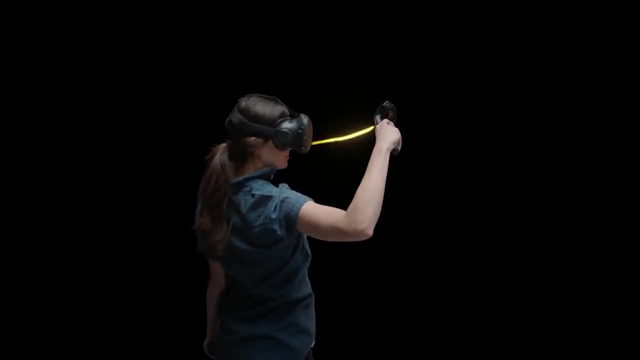 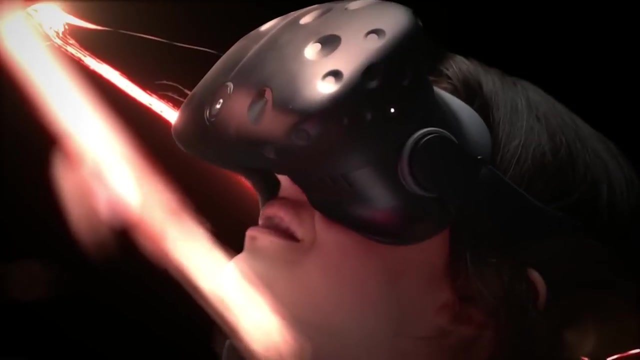 let's talk art class. Tilt Brush is an amazing artistic tool that lets you paint and create 3D art in VR. This experience is stunning, to be honest, and the only limit is the creativity of the person using it. If you're looking for a way to unleash creative energy, then this is one of the 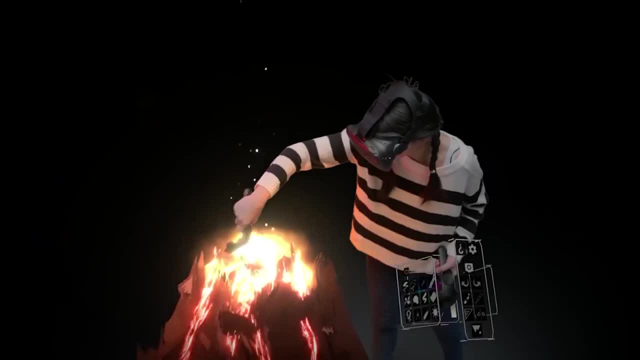 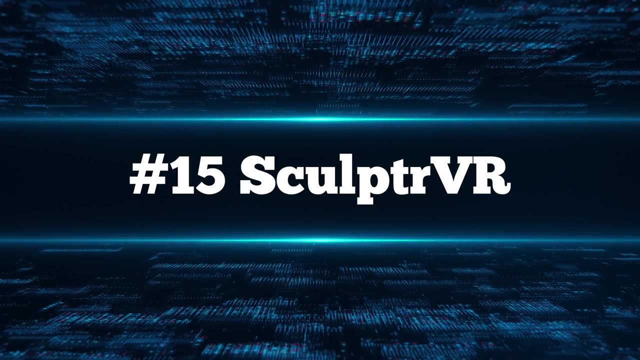 best ways to do it with many different brush types and features, plus the ability to walk through the art you've created is a totally new experience. Tilt Brush is $19.99.. Number 15, Sculpture VR. If you're looking to go a different direction for art, then check out Sculpture VR. This experience. 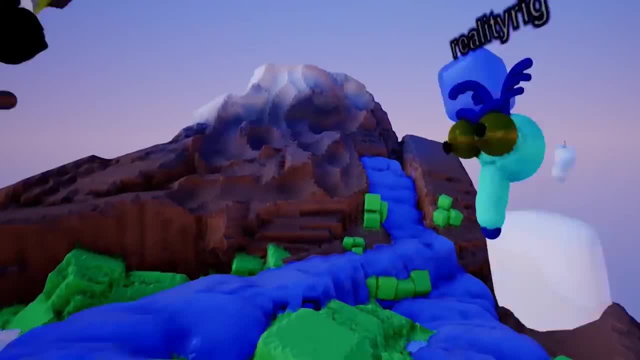 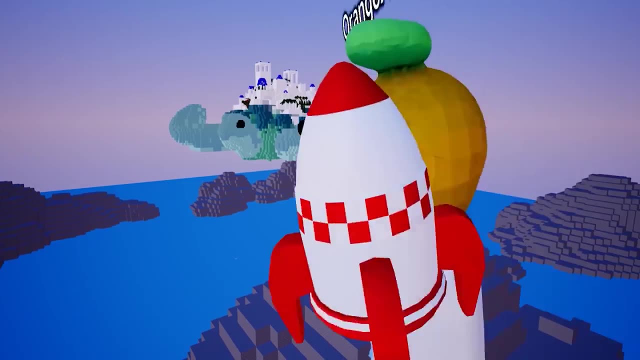 allows you to sculpt and create until your heart's content and with its amazing zoom and scale features, you can even do tiny details and then hand glide over your creations. Sculpture VR is $9.99.. Number 16, Other Various VR Videos, On top of all of the applications and 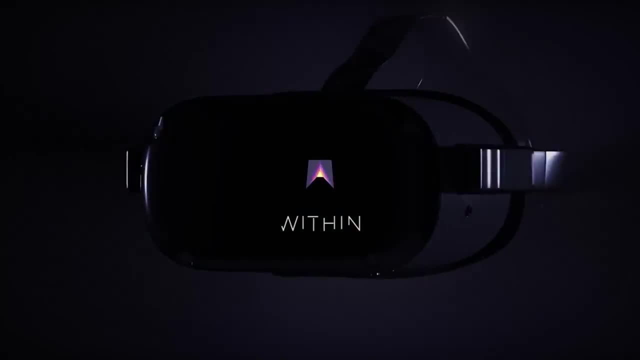 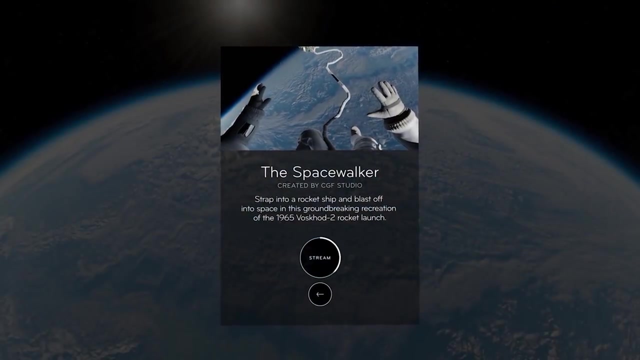 games mentioned above. there are a ton of educational 360 degree videos and 180 degree VR videos available on various platforms like Within, a curated application on the Quest that gives you some of the best VR videos, from education to entertainment, or Adam Savage's